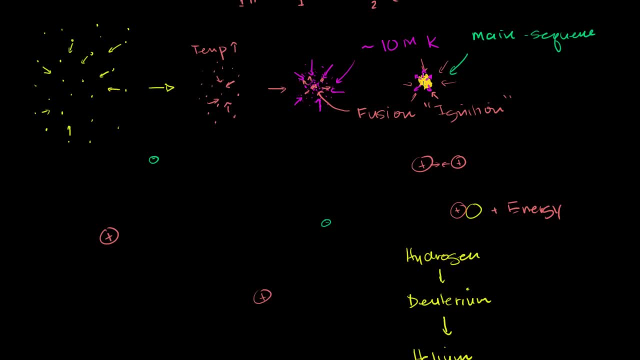 And then that energy begins to offset the actual gravitational force so that the whole star, what's now a star, does not collapse on itself. And once we're there, we're now in the main sequence of a star. What I want to do in this video is: 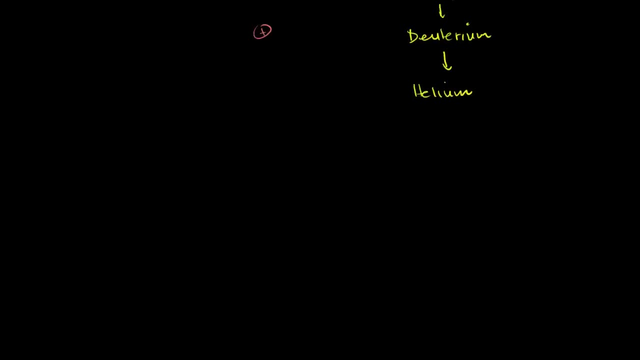 to take off from that starting point and think about what happens in the star next. So in the main sequence, we have a star, We have the core of the star. So this is the star's core And you have hydrogen fusing into helium. And it's releasing just a ton of energy, And that energy is what keeps the core from imploding. It's kind of the outward force to offset the gravitational force that wants to implode everything, that wants to crush everything. And so you have the core of a star, a star like the sun. 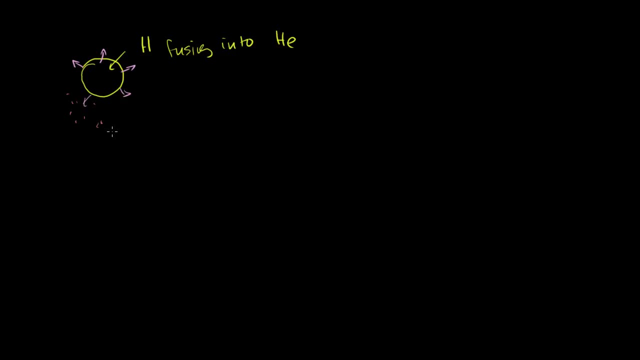 And that energy then heats up all of the other gas on the outside of the core to create that really bright object that we see as a star, or, in our sun's case, the sun Now, as the hydrogen is fusing into helium, 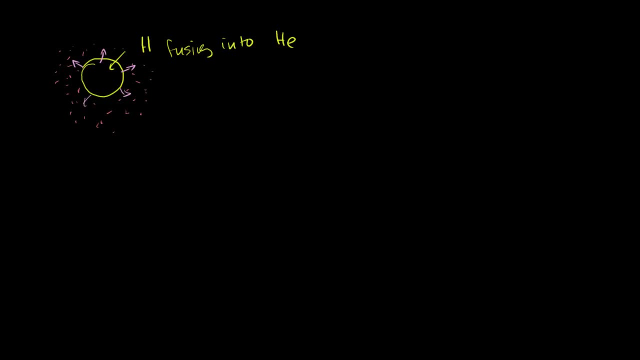 you can imagine that more and more helium is forming in the core. So I'll do the helium as green. So more and more helium forms in the core, It will especially form. the closer you get to the center, the higher the pressures will be and the faster that this fusion, this ignition, will happen. In fact, the bigger the mass of the star, the more the pressure, the faster the fusion occurs. And so you have this helium building up inside of the core as this hydrogen in the core gets fused. 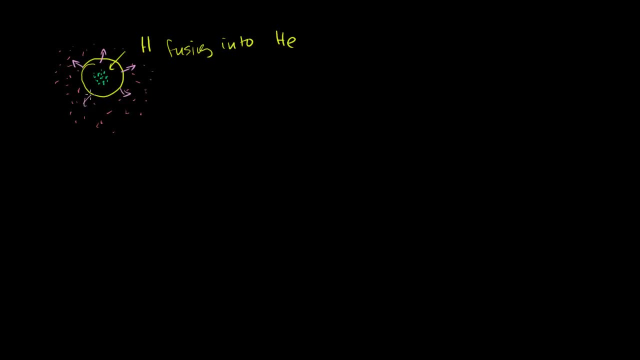 Now what's going to happen there? Helium is a more dense atom. It's packing more mass in a smaller space. So as more and more of this hydrogen here turns into helium, what you're going to have is the core itself is going to shrink. 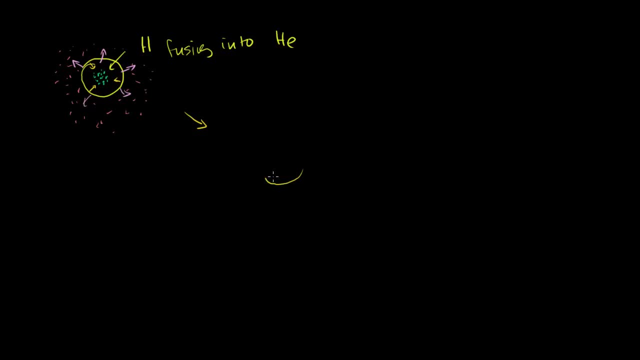 So let me draw a smaller core here. So the core itself is going to shrink And now it has a lot more helium in it, And let's just stick it to the extreme point where it's all helium, Where it's depleted, But it's been shrinking. 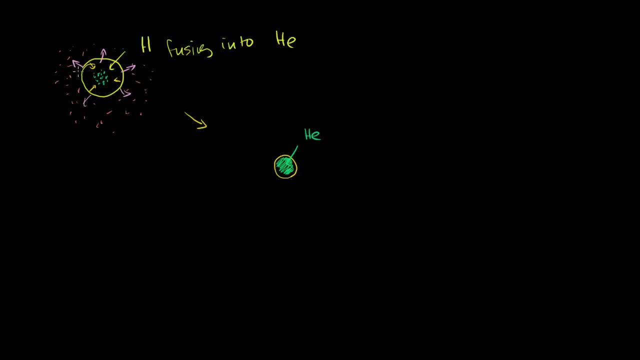 It's much denser. That same amount of mass that was in this sphere is now in a denser sphere, in a helium sphere. So it's going to have just as much attraction to it- gravitational attraction- But things can get even closer to it. 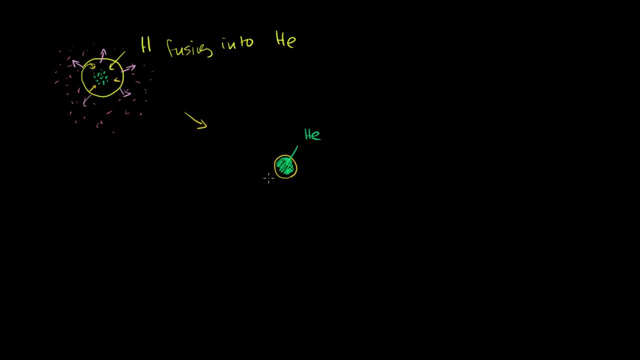 And we know that the closer you are to a mass, the stronger the pull of gravity. So then, instead of having just the hydrogen fusion occurring at the core, You're now going to have a small core, You're going to have hydrogen fusion in a shell. 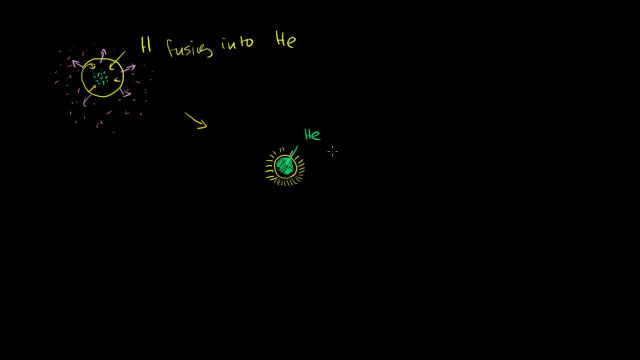 around the core. So now you're going to have hydrogen fusing in a shell around the core. Let me just be clear. This isn't just happens all of a sudden. It is a gradual process As we have more and more helium in the core. 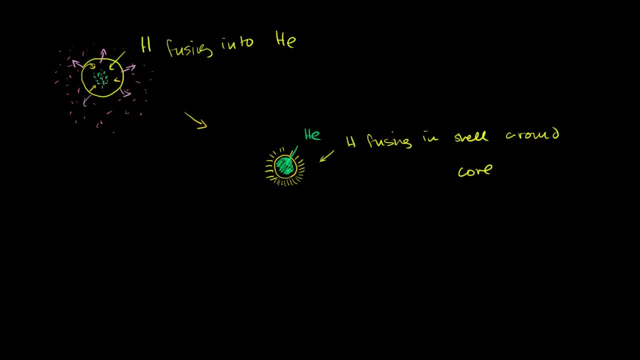 the core gets denser and denser and denser, And so the pressures, The pressures become even larger and larger near the core, Because you're able to get closer to a more massive core, since it is now more dense And as that pressure near the core increases even more. 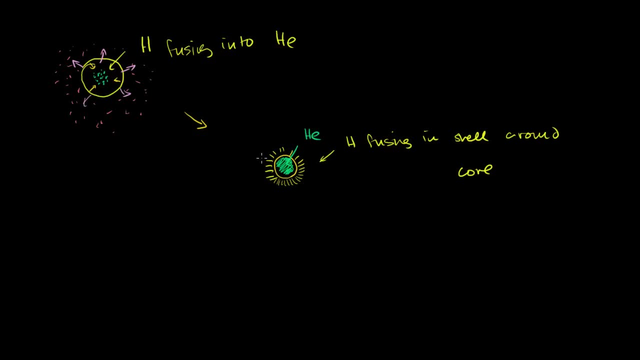 and more. the fusion reaction happens faster and faster and faster, until you get to this point. So here let me be clear. You have a helium core, All of the hydrogen in the core has been used up, And then you have the hydrogen right outside of the core. 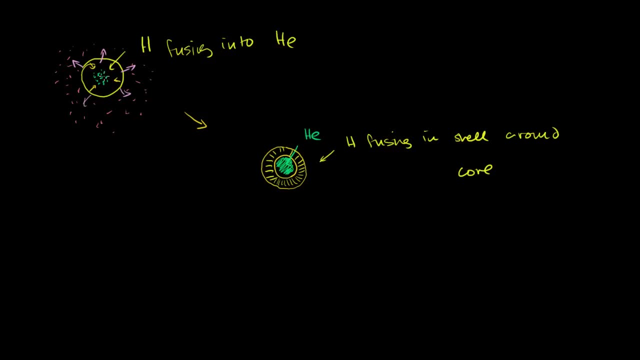 is now under enormous pressure. It's actually under more pressure than it was when it was just a pure hydrogen core Because there's so much mass on the outside here trying to- I guess you could say exerting downward or gravitational force- trying to get to that even denser helium core. 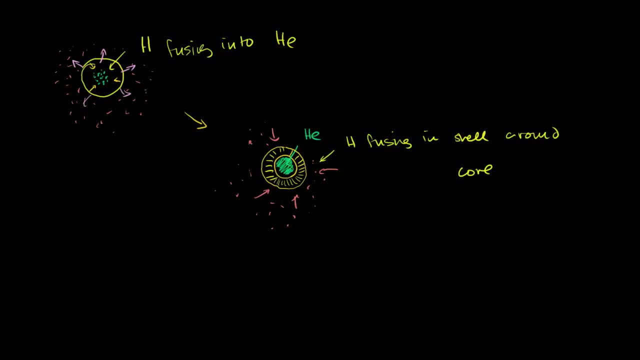 Because everything is able to get closer in, And so now you have fusion occurring even faster, And it's occurring over a larger radius. It's occurring over a larger radius, So this faster fusion over a larger radius is then going to. the force is now. 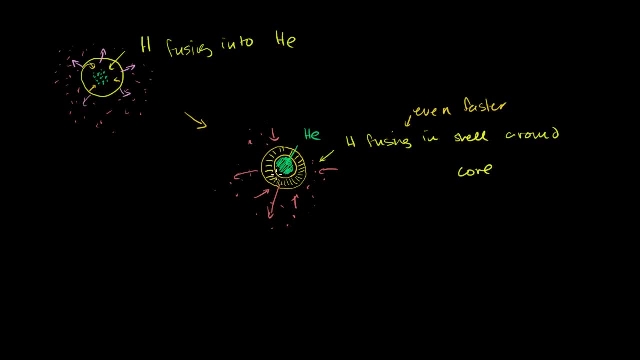 going to expel the energy that's released from this fusion is now going to expel these outer layers of the star even further. So the whole time, this gradual process as the hydrogen turns into helium or fuses into helium in the core. 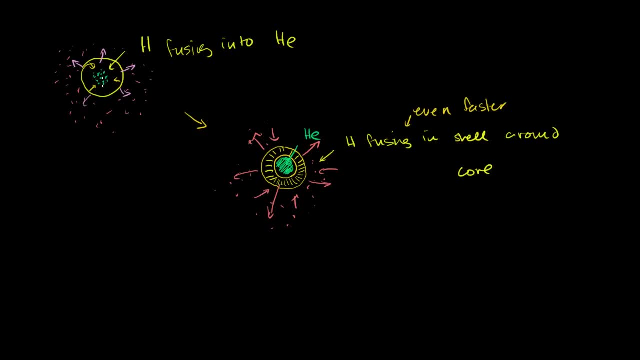 the hydrogen right outside of the core, right outside of that area, starts to burn faster and starts to- or I shouldn't say burn, it starts to fuse faster and faster over a larger and larger radius. So the unintuitive thing is the fusion. 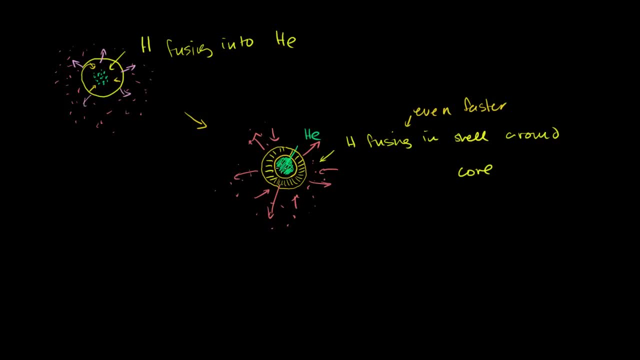 is happening faster, over a larger radius, And the reason that is is because you have even a denser core. that is causing even more gravitational pressure And as that's happening, the star is getting brighter, And it's also the fusion reactions. 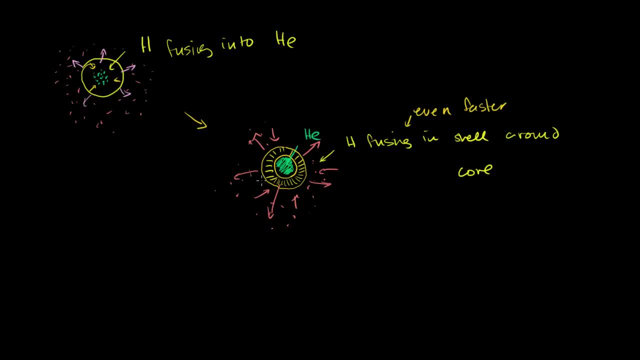 since they're happening in a more intense way and over a larger radius, are able to expel the material of the star even larger. So the radius of the star itself is getting bigger and bigger and bigger. So if this star would look like this, if this star 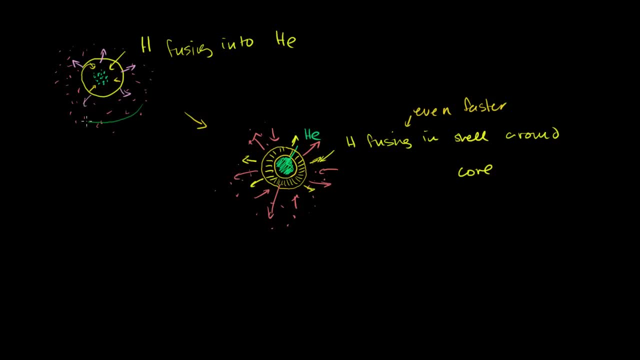 maybe let me draw it in white. This star looked like this. That's not white. This star looked like what's happening to my color changer. There you go, OK. this star looked like this right over here. Now this star over here since a faster fusion reaction. 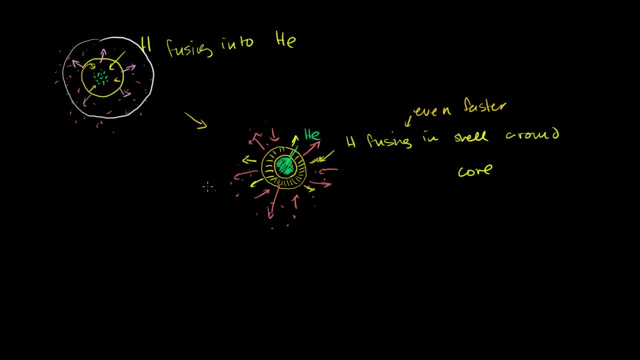 is happening over a larger radius is going to be far larger, And I'm not even drawing it to scale. In the case of our sun, when it gets to this point, it's going to be 100 times the diameter And at this point it is a red giant. 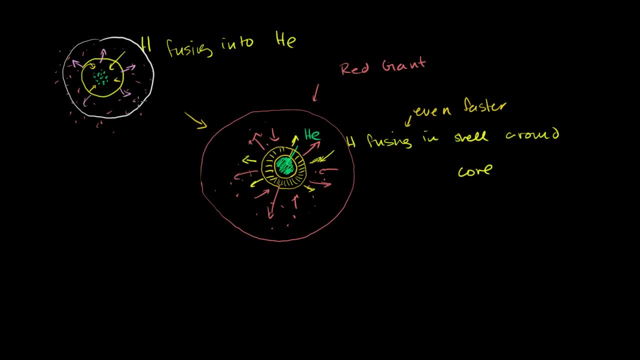 And the reason why it's redder than this one over here is that, even though the fusion is happening more furiously, that energy is being dissipated over a larger surface area. Let's see. So the actual surface temperature of the red giant at this point is actually going to be cooler. 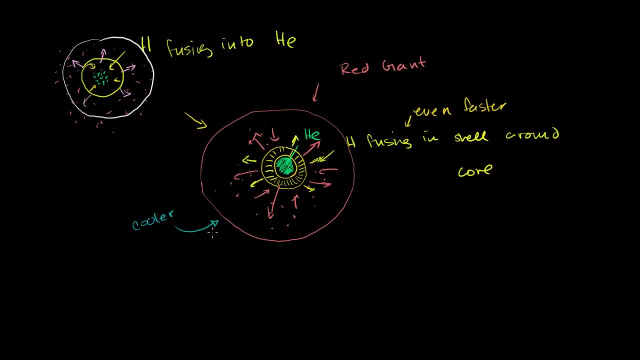 So it's going to emit a light at a larger wavelength, a redder wavelength than this thing over here. This thing, the core- was not burning as furiously as this thing over here, But that energy was being dissipated over a smaller volume. 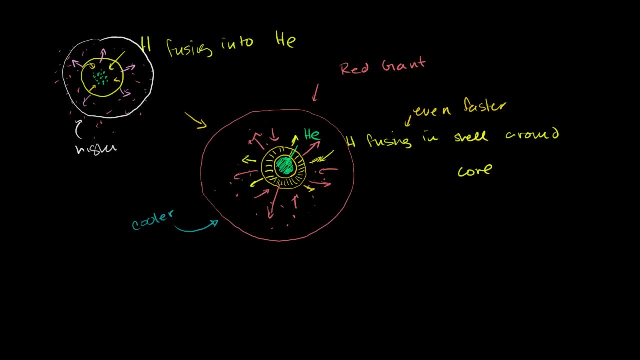 So this had a higher surface temperature. This over here, the core is burning more. Sorry, the core is no longer burning. The core is now helium. that's not burning. It's getting denser and denser as the helium packs in on itself. 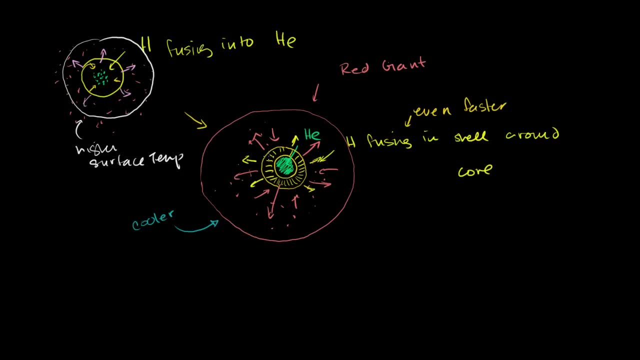 But the hydrogen fusion over here is occurring more intensely. It's occurring in a hotter way, But the surface here is less hot because it's just a larger surface area. So it doesn't make. the increased heat is more than mitigated by how large the surface area is. 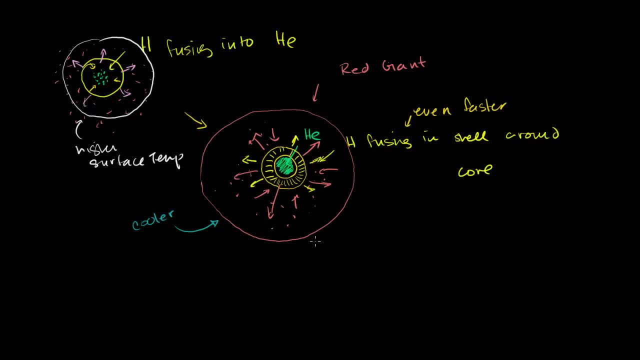 So it's getting denser and denser as the helium packs in on itself. It's getting larger and larger as the star has become. Now this is going to keep happening, keep happening, And this core, the pressures, keep intensifying because more and more helium is getting produced. 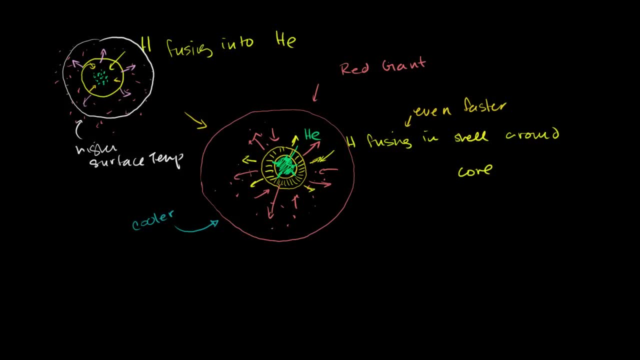 And this core keeps collapsing And the temperature here keeps going up. So we said that the first ignition, the first fusion, occurs at around 10 million Kelvin. This thing will keep heating up until it gets to 100 million Kelvin, And now I'm talking about a star that's about as massive as the sun. 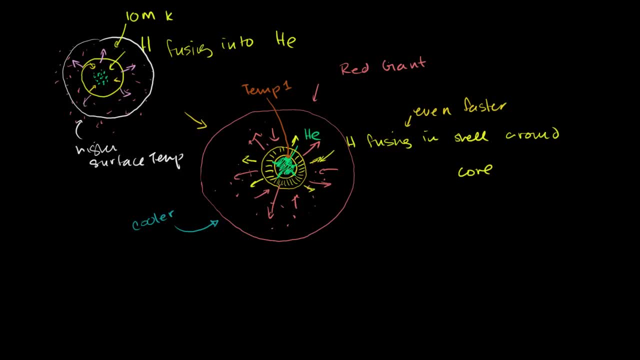 Some stars will never even be massive enough to condense the core so that its temperature reaches 100 million, But let's just talk about the case in which it does So. eventually you'll get to a point. So we're still sitting in the red giant phase. 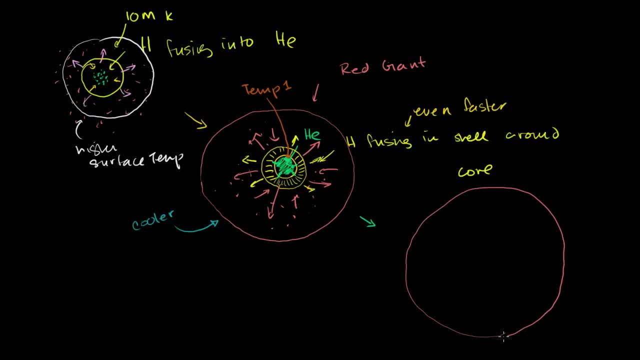 So we're this huge star over here. We have this helium core. That helium core keeps getting condensed and condensed and condensed, And then we have a shell of hydrogen that keeps fusing into helium around it. So this is our hydrogen shell. Hydrogen fusion is occurring in this yellow shell over here. 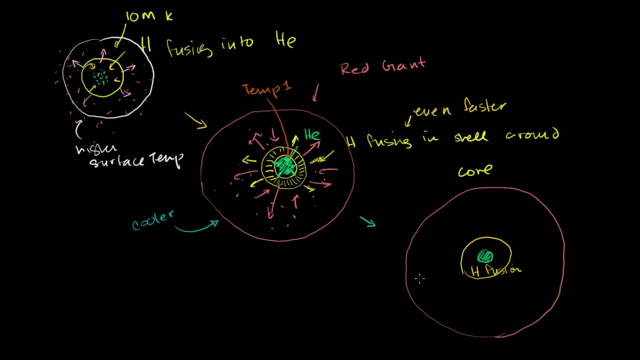 that's expelling, that's causing the radius of the star to get bigger and bigger, to expand, But when the temperature gets sufficiently hot- and now I think you're going to get a sense of how heavier and heavier elements form in the universe- 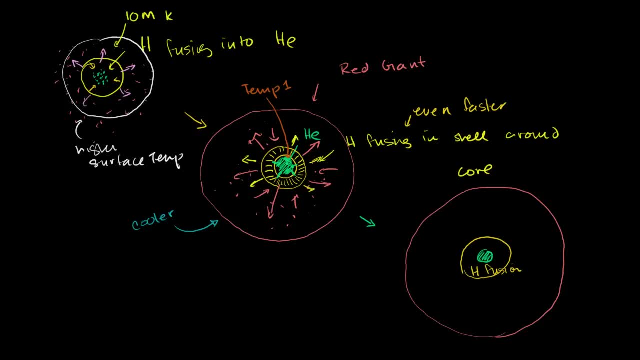 And all of the heavy elements that you see around us, including the ones that are in you, are formed this way: from initially hydrogen, When it gets hot enough, at 100 million Kelvin. 100 million Kelvin in this core because of such enormous pressures. 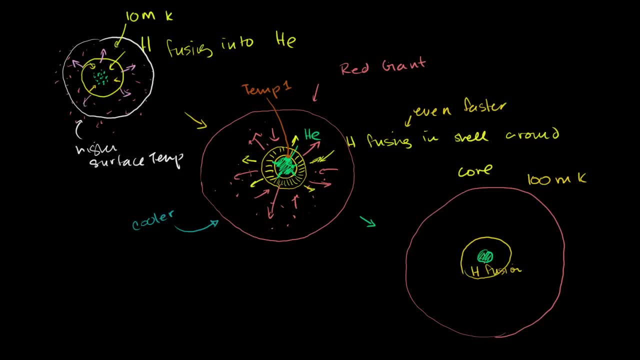 then the helium itself will start to fuse. So then we're going to have a core in here where the helium itself will start to fuse. The helium will start to fuse. And now we're talking about a situation: you have helium and you have hydrogen. 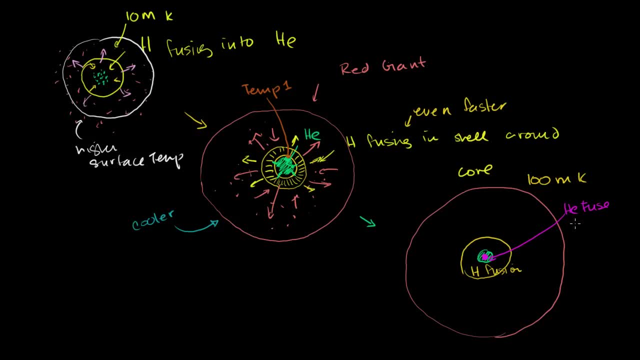 all sorts of combinations will form, But in general the helium is mainly going to fuse into carbon and oxygen And it will form into other things and it becomes much more complicated. but I don't want to go into all of the details. 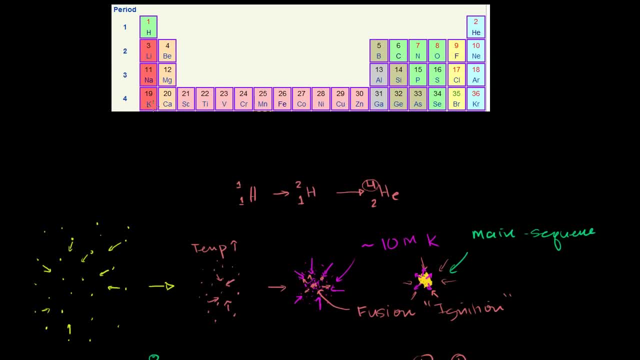 But let me just show you a periodic table. I didn't have this in the last one, I somehow had lost it. But we see, hydrogen here has one proton. It actually has no neutrons. It was getting fused in the main sequence into helium: two protons, two neutrons.